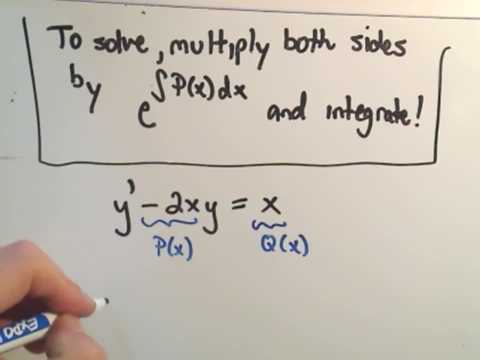 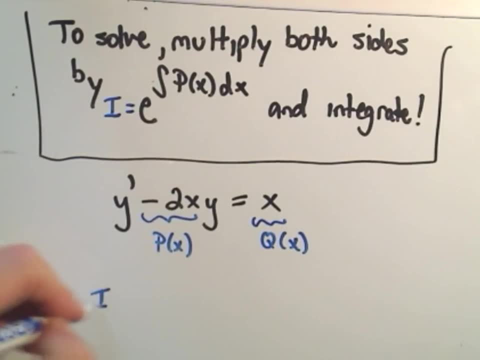 So it seems a little strange, but it's a technique that works. So really, it says: to find this. they sometimes call this the integrating factor. so to find this integrating factor, we'll take e and raise it to the negative 2x power. 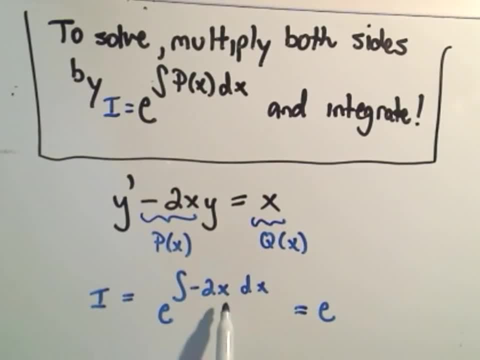 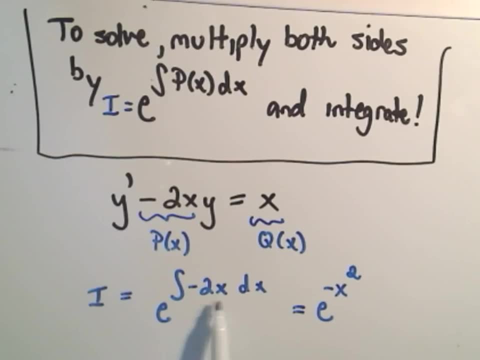 dx. Well, if we integrate negative 2x, we'll just get negative x squared. Okay, so if you integrate negative 2x, we simply get negative x squared. And it says: this is what we're going to have to multiply both sides of our equation by. 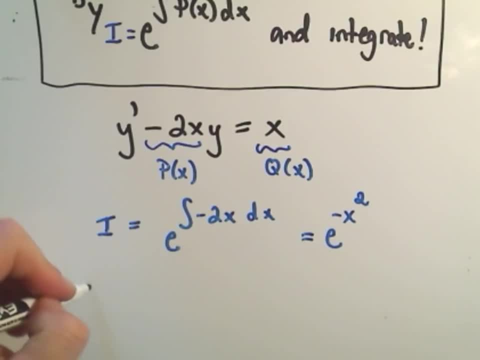 So okay, well, let's do that. So on the left side, I'm going to get e to the negative x squared Times y prime minus 2xy, And then this will be equal to x times e to the negative x squared. 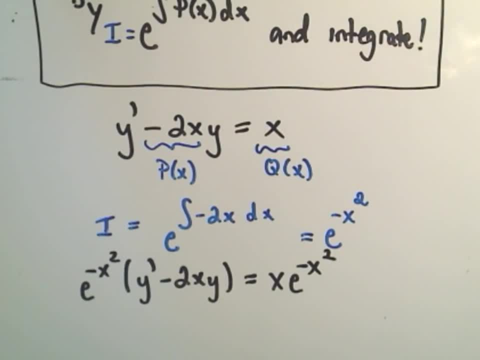 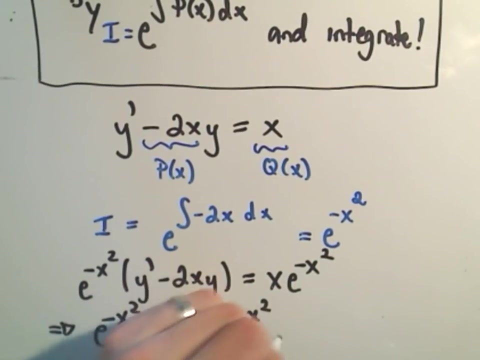 And what we have to do now is we have to multiply both sides or again, integrate both sides. excuse me, Notice, if we multiply this out, the left side too, we'll get e to the negative x squared times, y prime plus 2x, e to the negative x squared y. 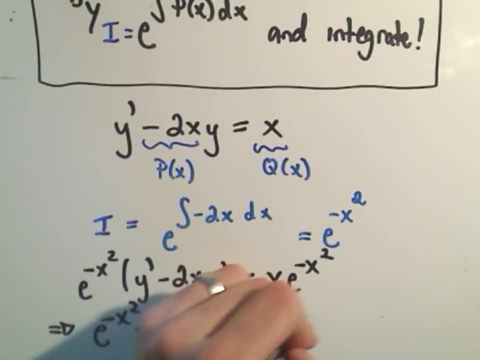 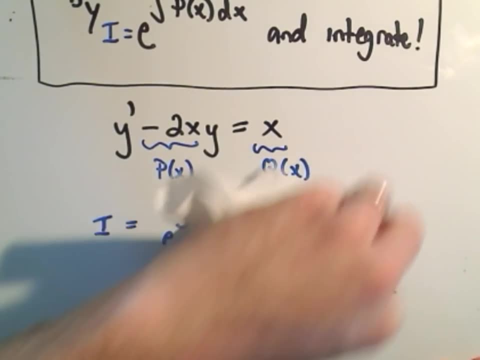 Okay, so I'm just distributing that term out And the right side, we'll leave alone: x e to the negative, x squared. Okay, so this is the thing that, again, I'm going to have to clean up and integrate here. 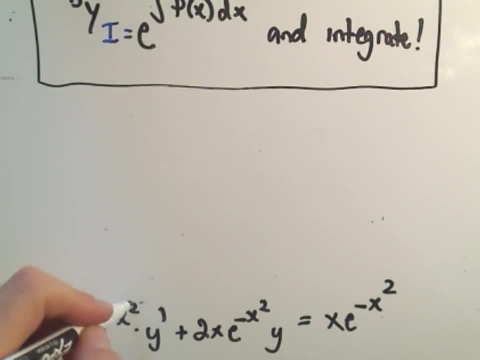 The key thing in this problem is: one of the key things is this left side. Okay. so again, we have to integrate both sides. That's what we're going to do now. I should tack a dx onto the left side as well. 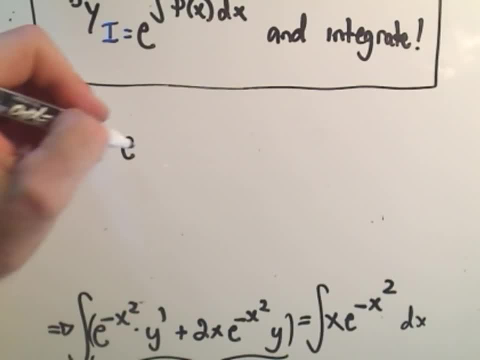 Notice, if you integrate, If you integrate the left side, you'll actually get that integrating factor e to the negative x squared times y. Okay, and take the derivative of this thing. If you take the derivative, what will you get? Well, you'll leave the first part alone. 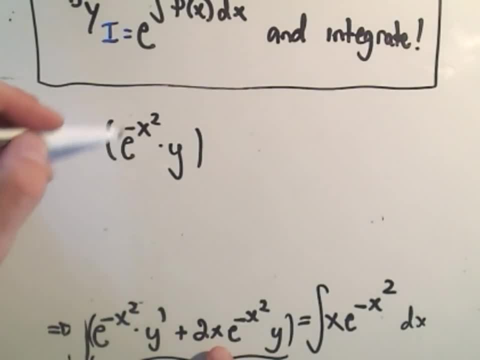 Then you'll get y prime, which is this part. Plus, if you take the derivative of e to the negative x squared, you'll get the 2x e to the negative x squared times y term. Okay, so this is the whole trick. 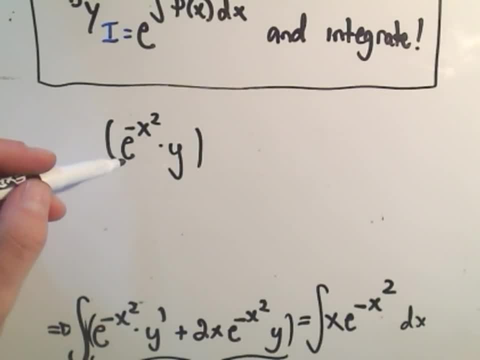 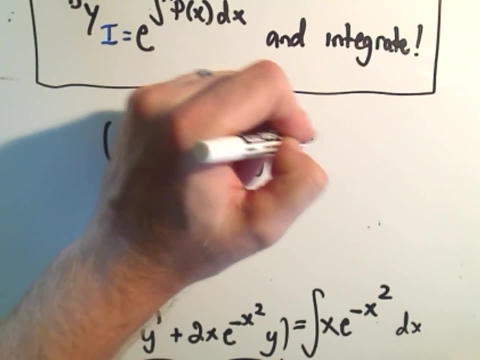 That if you integrate the left side, You just get your integrating factor times y Okay. we still do have to integrate the right hand side, though, So that one will be a touch- well, a touch trick here. I guess Not too much work. 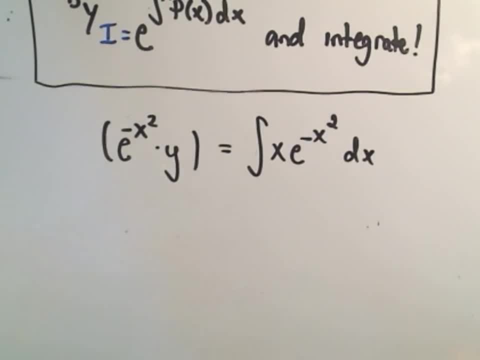 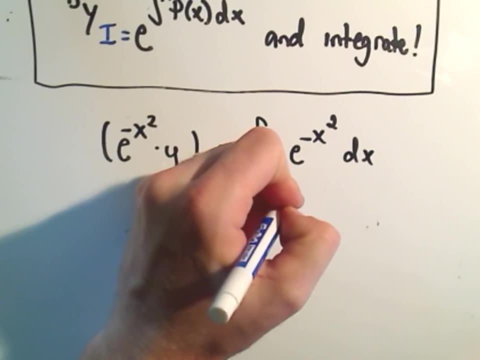 This is again the only one that you'll really have to. you know, think about or use your integration techniques on. So on the right side, we can just do this with a u substitution. It says: if we let u be negative x squared, well, then du will be negative 2x. 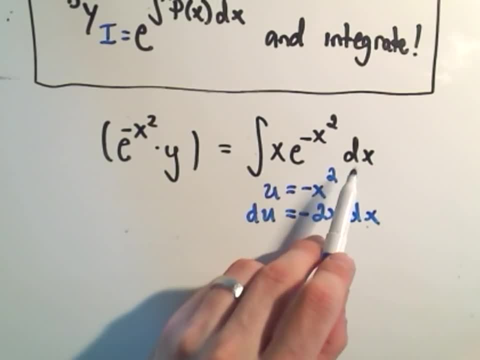 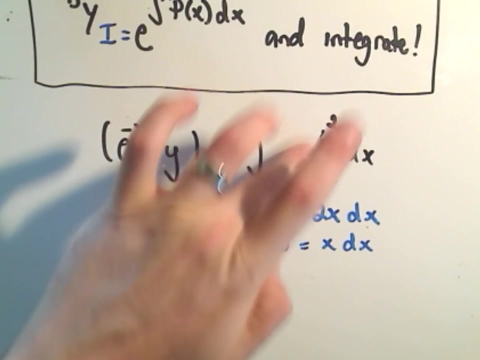 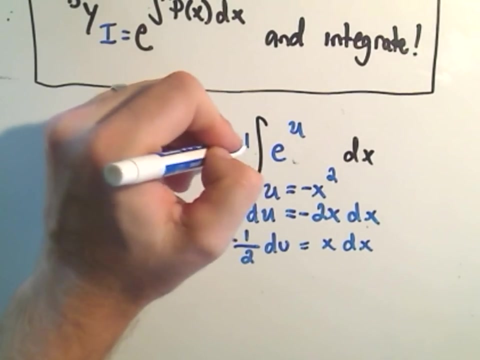 Okay, the way I think about it is: we want to replace an xdx. so if I divide both sides by negative 2, I'll get negative 1 half. du equals xdx. So then if I integrate that, if I relabel all of that, the e to the negative, x squared will turn into the e to the u and then the xdx that's left over. I can take the 1 half and my dx will now turn into a du. 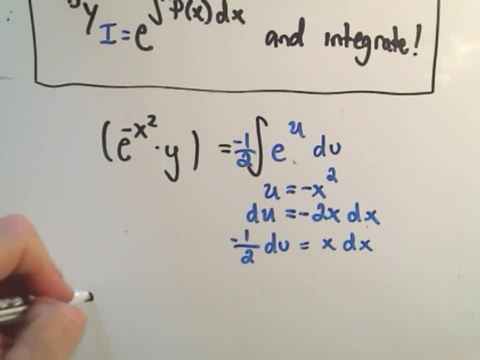 Okay, so again we're done with the left side. We've actually already integrated that side. On the right side we'll get negative 1 half e to the u, but again we know that u is negative x squared plus c. 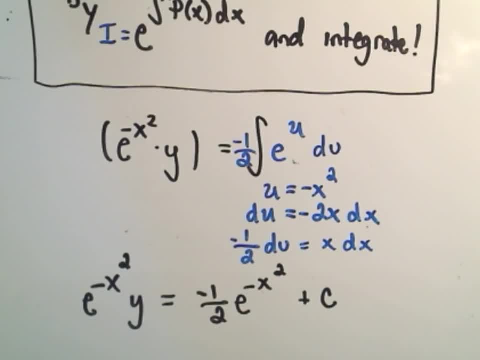 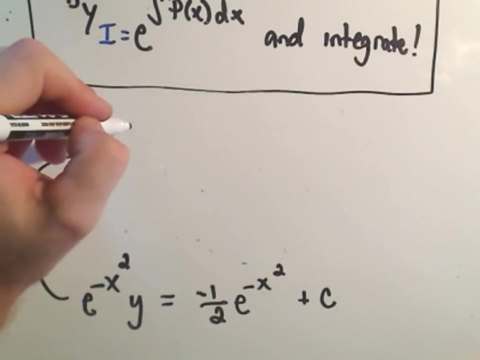 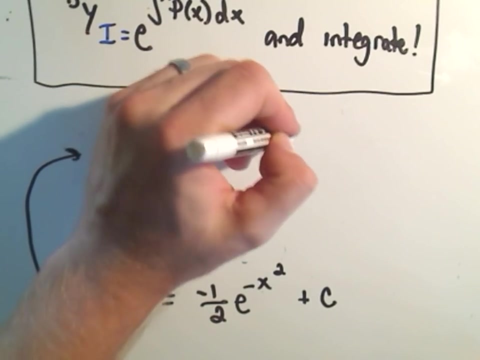 And at this point, technically, you've got your solution here, So you could always even go ahead and divide both sides, I guess, just to get your y term alone. So we can do that real quick. It says that we'll simply get: hey, just divide both sides, we'll get. y equals negative 1 half e to the negative x squared, plus c divided by e to the negative x squared. 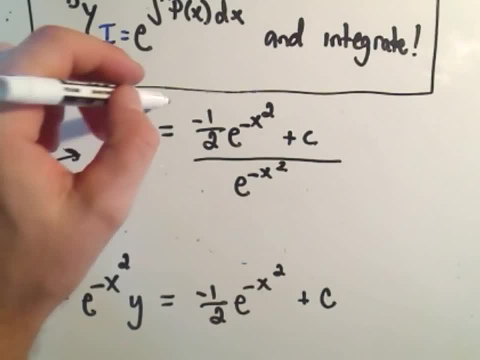 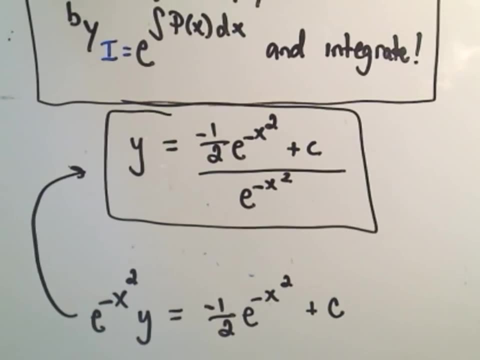 And of course we could clean this up a little bit further, but I'm going to be lazy and stop right there. If you're looking at stuff about differential equations, I assume that your algebra is problematic. It's probably okay to clean that up a little bit. 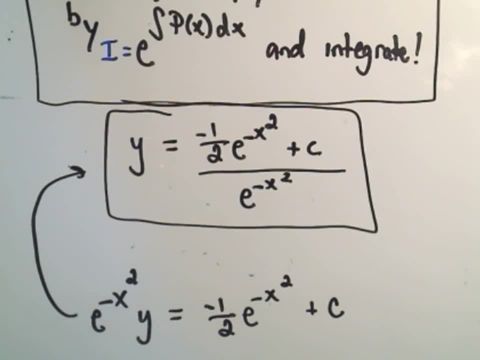 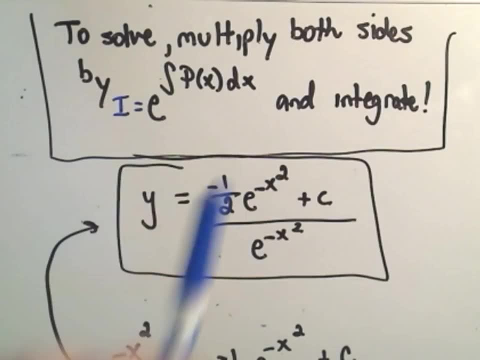 So all right, this is the basic idea with these first-order linear differential equations. Again, you multiply by this integrating factor on the left side. So you take e and raise it to the p of x, And again, when you integrate the left side you'll get that integrating factor times y.